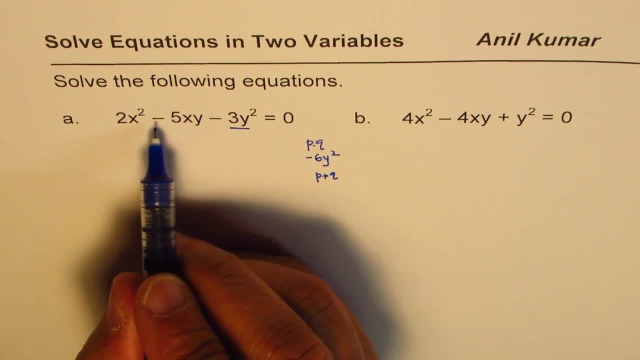 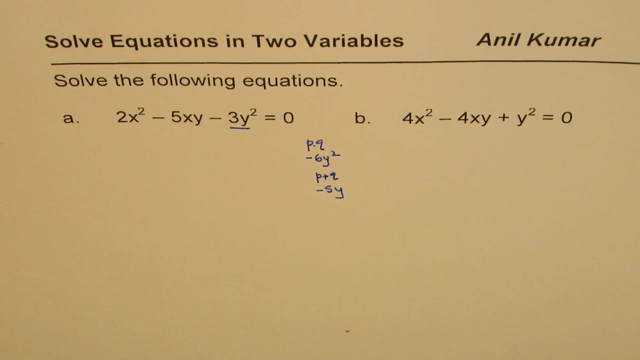 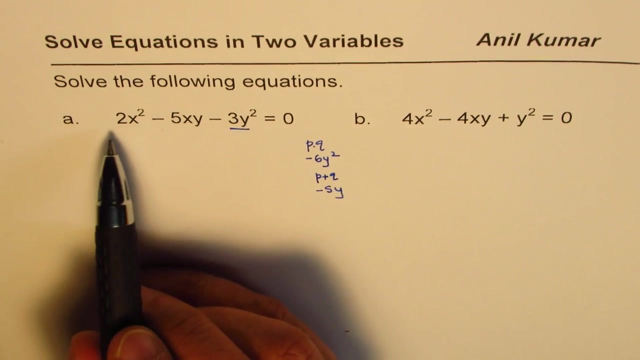 And we want the sum p plus q as the middle number, minus 5y, minus 5y, Think like that. So product of 2 times 3y squared. We know we have a minus. Now we know we have a 3y squared, So we want the sum p plus 3y squared. 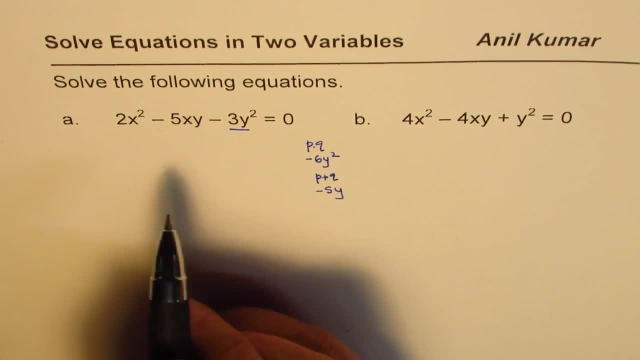 That is minus 6y squared And sum of minus 5y. Now what numbers could satisfy this? We know 6x squared is 1.. We know x equals 3y squared. We know x equals 3y squared is 1.. 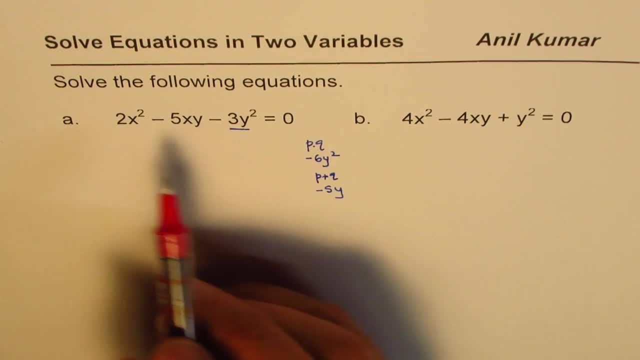 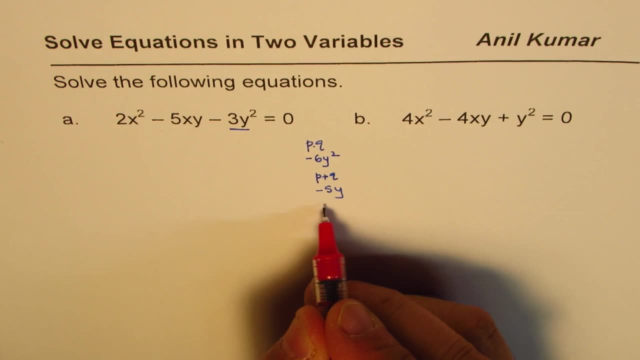 We know y equals 3y squared. We know y equals 3y squared is 1.. times 1 is 6, we need minus and therefore the two numbers are of opposite sign. So the numbers could be 6y minus 6y and y. So if I add them I get minus 5y. Do you get? 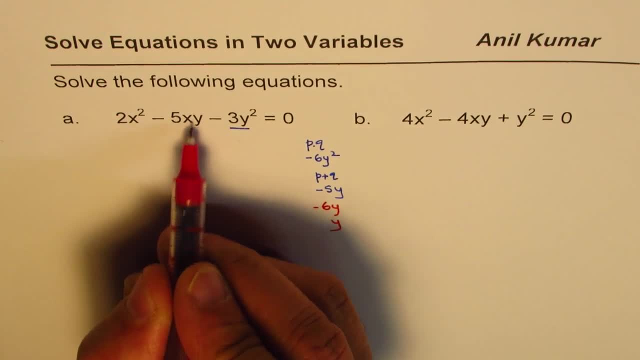 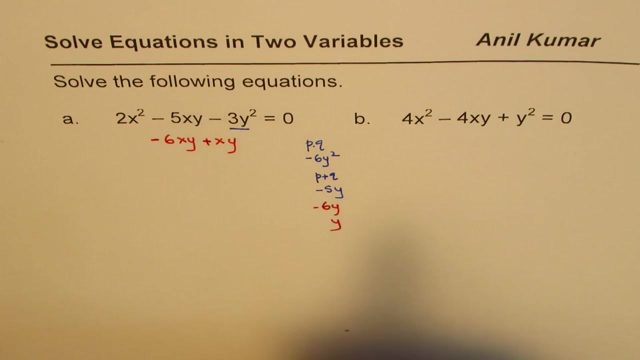 the idea. So we'll split this minus 5xy as minus 6xy, and y I mean plus xy. Do you understand? So x is a variable now. So we are looking as if we are working with a single. 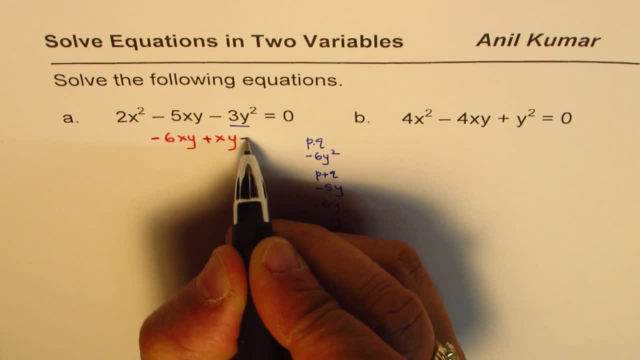 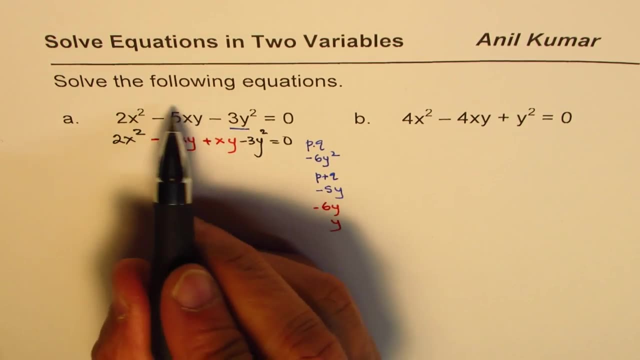 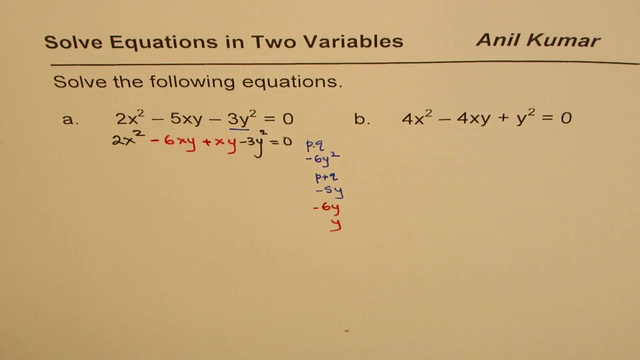 variable. So that really helps. The rest of the things are: 3y squared equals to 0, and we have 2x squared. So basically, we'll split the middle, We'll split the middle term, as we did for most of the factoring examples. And now you. 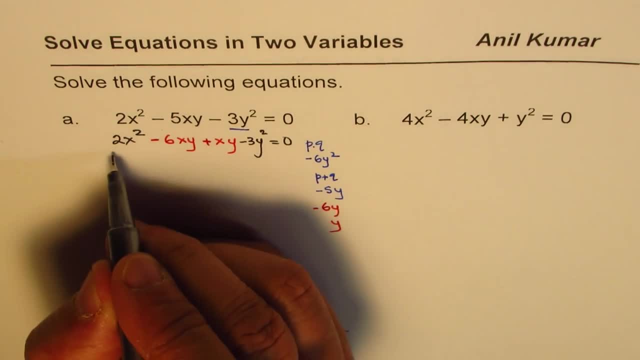 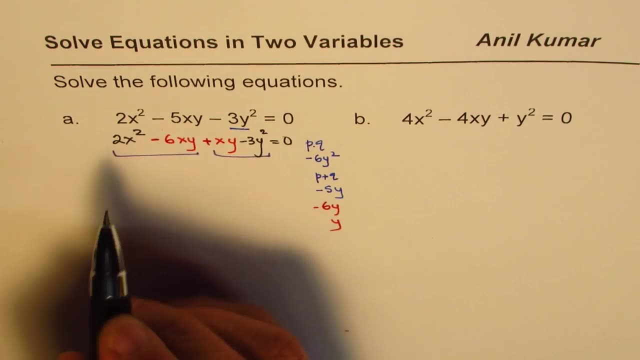 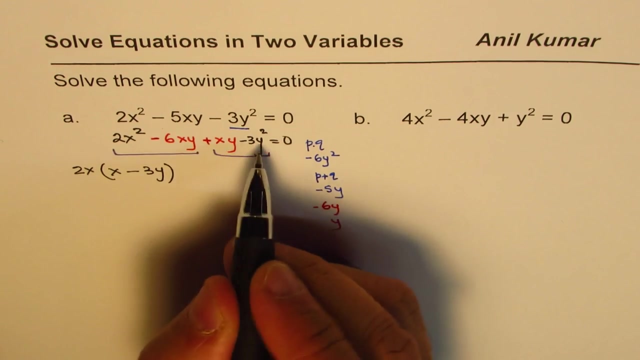 can combine the first two and the last two, right, So you can combine these two and these two. What is common? 2x is common here, So we can say 2x and we get x minus 3y In this. 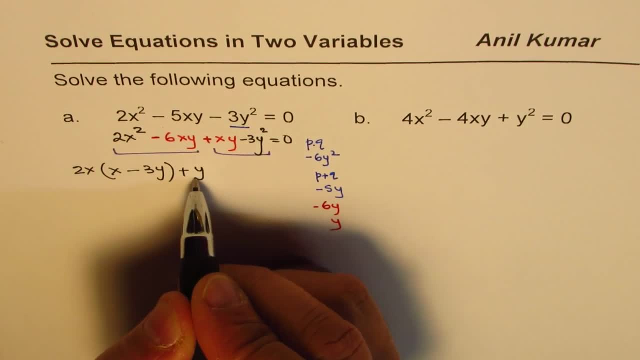 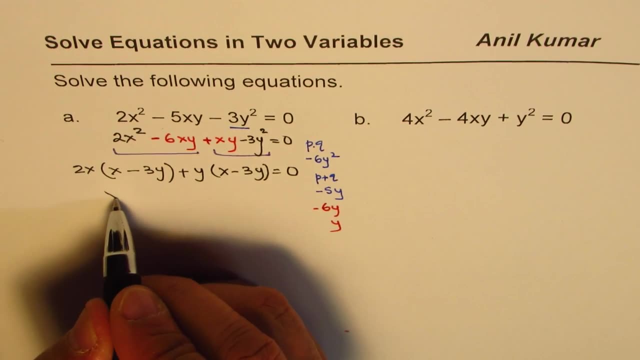 case, what is common? y is common, and we get x minus 3y. So we get x minus 3y. So x minus 3y equals to 0.. Now x minus 3y is common, So we write x minus 3y, We're left. 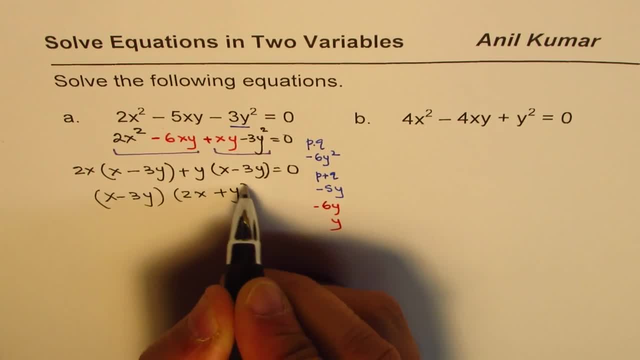 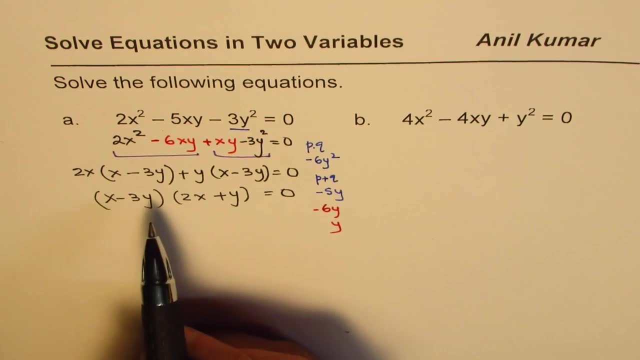 with 2x plus y equals to 0.. So that is the factored form. Once you get to the factored form, then equate each factor to 0, which will give you two different solutions. right? So from here we are looking for solutions now. 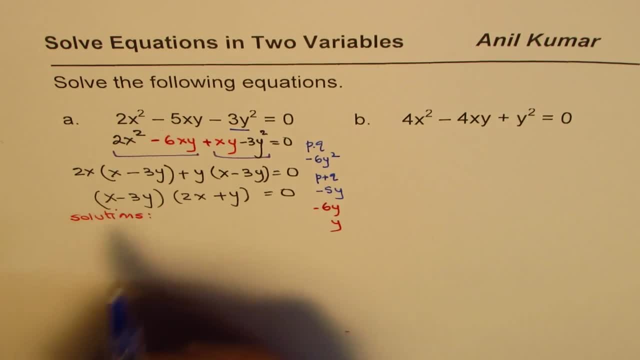 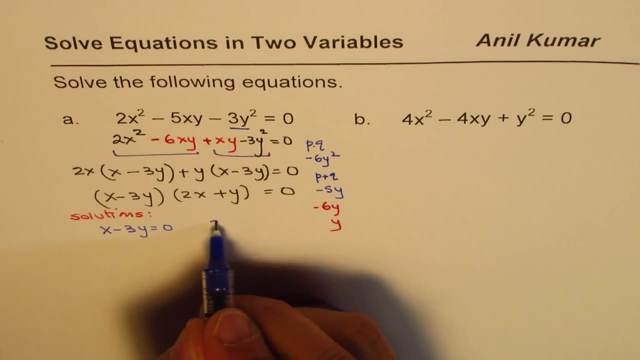 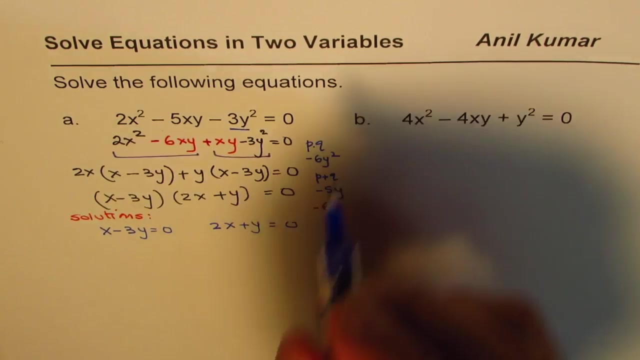 How Equate each factor to 0. So we can write: x minus 3y equals to 0.. Solve for x. And we can equate: 2x plus y equals to 0.. Solve for x. okay, So that is what it is, So basically. 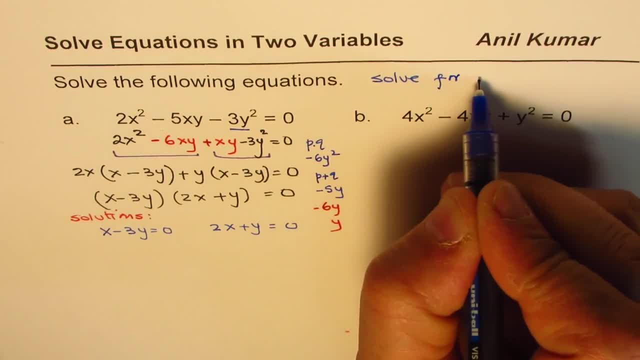 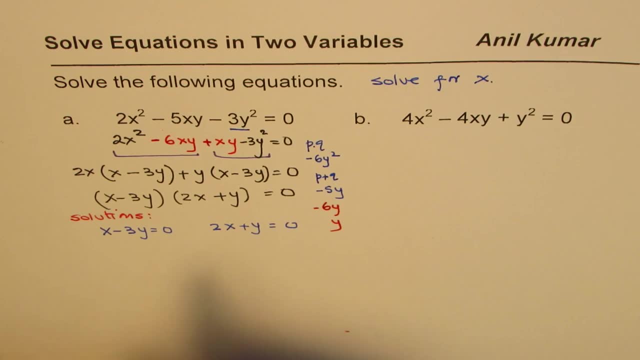 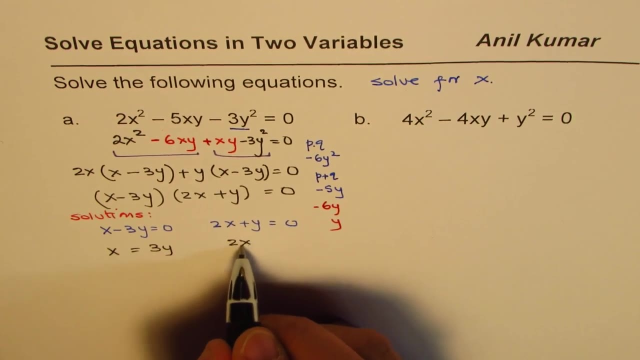 we'll solve for x. So we'll treat this equation, which may have two variables, as the equation in one variable, x. okay, So let's solve. So we get x equals to 3y, And here what do we get? We get 2x equals to minus y, or? 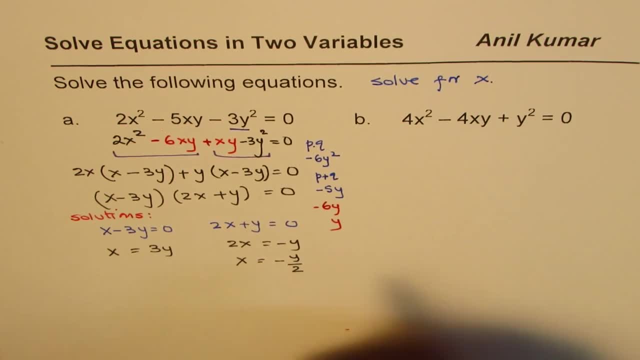 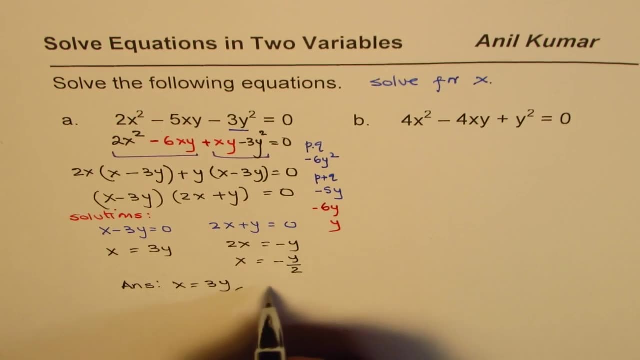 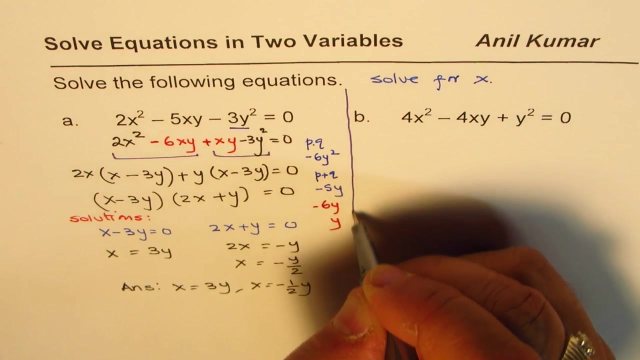 x equals to minus y over 2, or half y. So we have two solutions. Our answer is x equals to 3y and x equals to minus half y. So I hope the steps are clear. So, basically even. 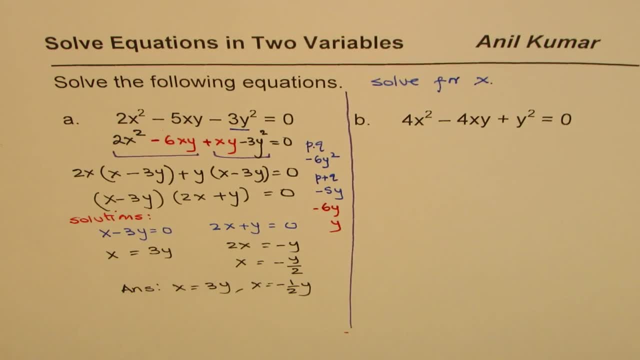 if the equation has two variables, treat it So we have one variable and apply the concepts which you have learned right. So here we applied the product and sum technique to factor, and then each factor should be equated to 0 to find the value of x. That's what we call solving equations, correct? Now let's do. 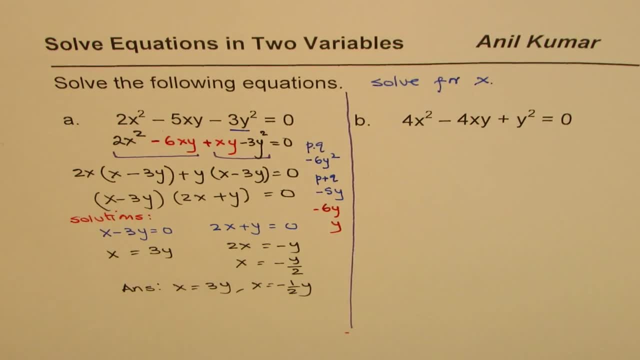 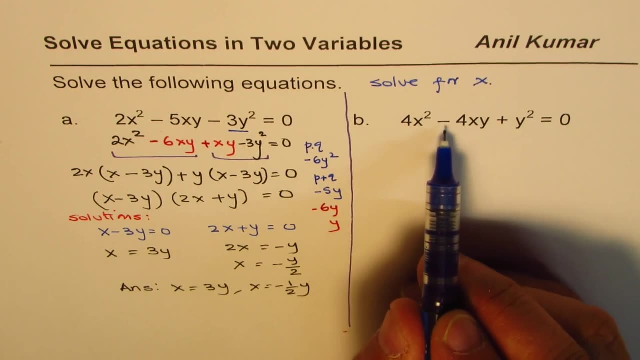 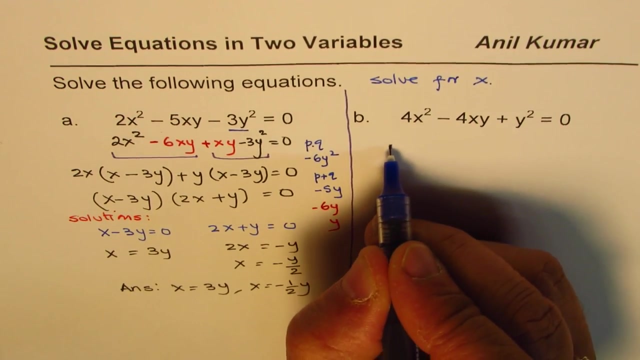 the next one. You can actually now pause the video, answer the question, solve this part and then look into my suggestions right Now. the second equation is: 4x squared minus 4xy plus 1y Y squared equals to 0. It seems to be a perfect square, See: 4x squared is 2x whole squared. 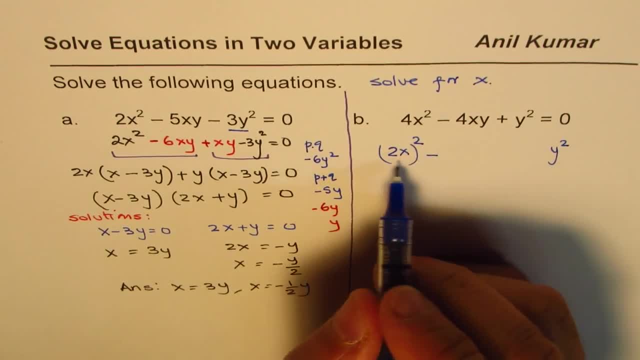 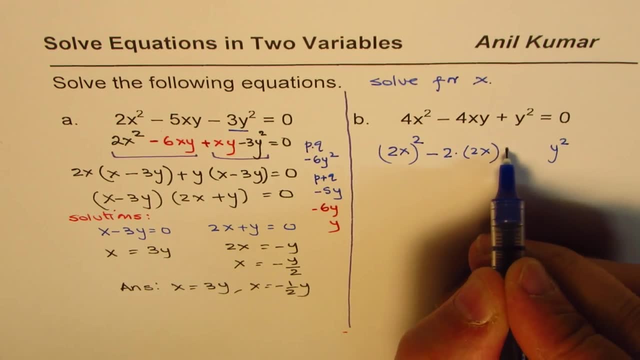 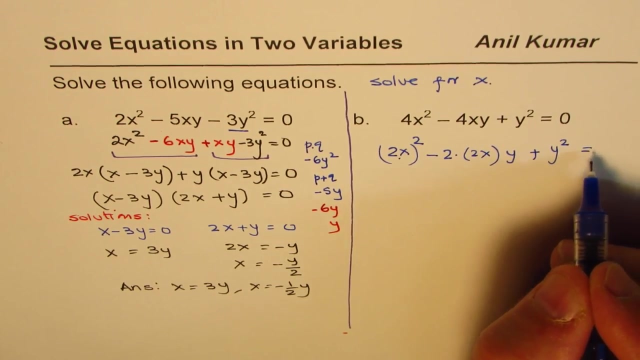 Y squared is y squared And the center term is minus 2 times 2x times y. Do you see that Here we have plus, So center term is twice the product of these two. right, And therefore we could actually write that equation as: 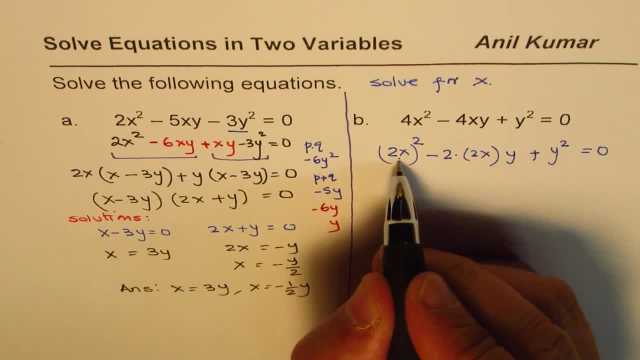 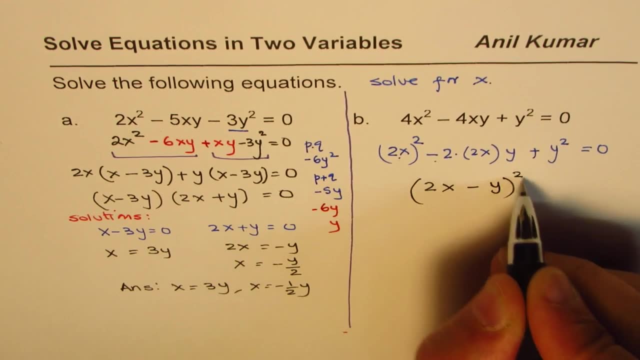 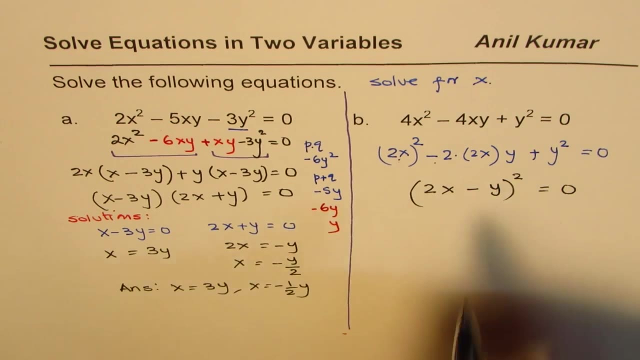 as 2x minus y whole squared. So we could factor this as 2x minus y, whole squared, equals to 0.. So since we recognized this equation as a perfect square, it was simple. You would always adopt this method of product and sum two, factor right. Well, here we have only.